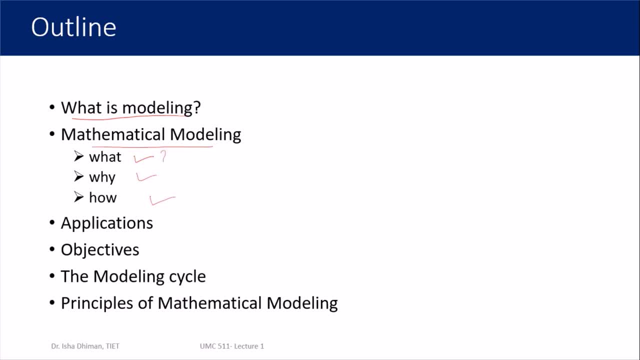 first lecture, I'll be definitely answering what it is and why it is, and the how part will be explained in the subsequent lectures. Let's first look at some of the interesting applications of mathematical modelling, followed by objectives of it, although there are no well-defined and fixed objectives, but yet. 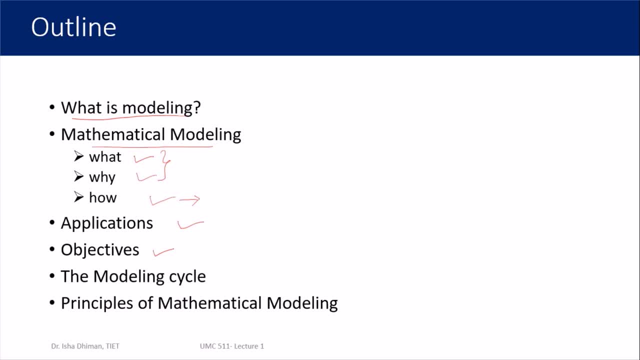 still we can discuss few of them. And then we'll begin with the definition of the modelling cycle and, in detail, we'll be discussing the principles of mathematical modelling. So let's explore all of these one by one. What is modelling? To understand the modelling process, we need to first understand the meaning of the word. 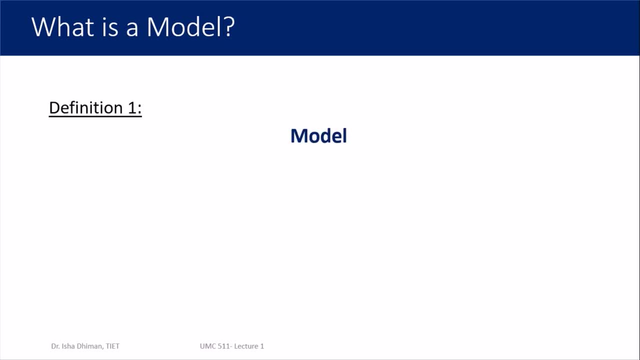 model. So first question is: what is a model? So I would suggest you to pause the video here and think about this word, that whatever comes to your mind whenever you look at the word model, you read it somewhere or you hear the word model anywhere. So a model is nothing. 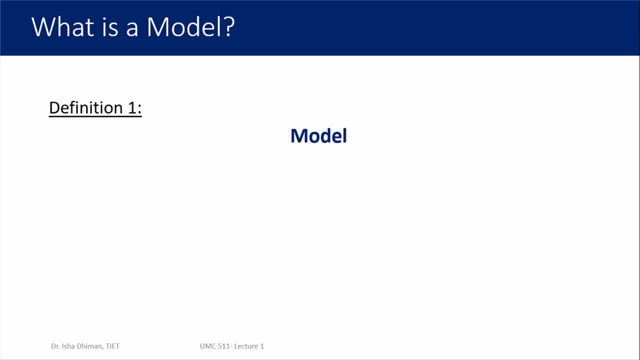 but a replication of something which is happening in real. So we can have few statements which can be considered as definitions of the model. A model is a miniature or abstract representation of something. Why it is called miniature? because most of the times the model is drawn on a small scale as compared to the real object. 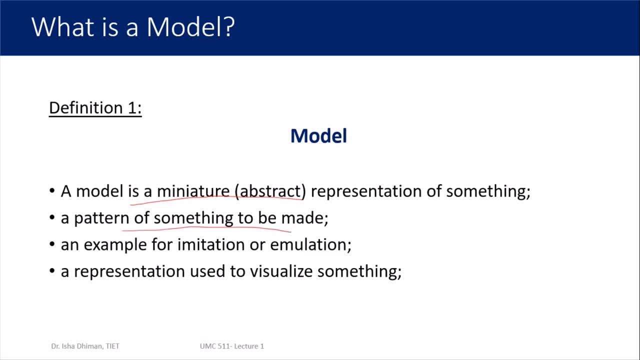 A pattern of something to be made. like we want to construct something, but before actual construction We want to understand it through the modelling process. so we'll draw its pattern or the diagrams. It can be an example for imitation. For example, you want to learn something, you want to see. 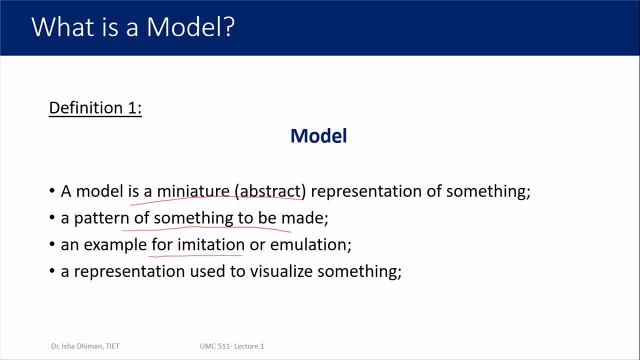 how the real object or the real phenomena is happening. So you will try to replicate it through modelling And it can be a representation used to visualize something. So, as I just told you, there is no well-defined definition. All of these are different ways of understanding the word model. 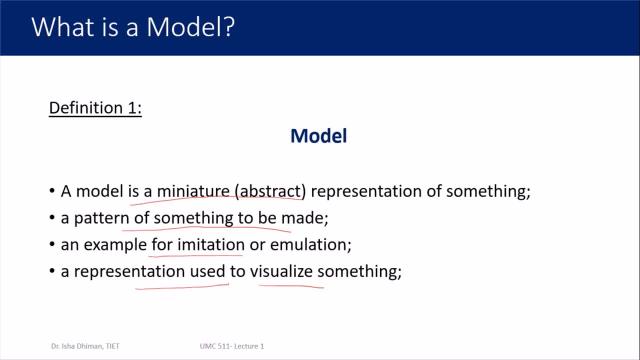 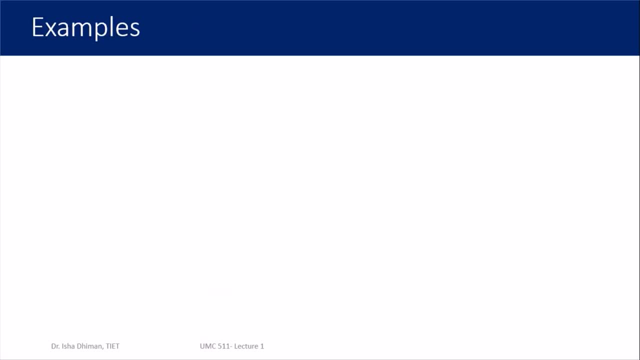 So, before moving to the specific mathematical model, I would like to give you some few examples of these models in general. So the first example we are going to look at is physical model, which is also known as prototype. So it's clear from the name that physical means something which you can see with your 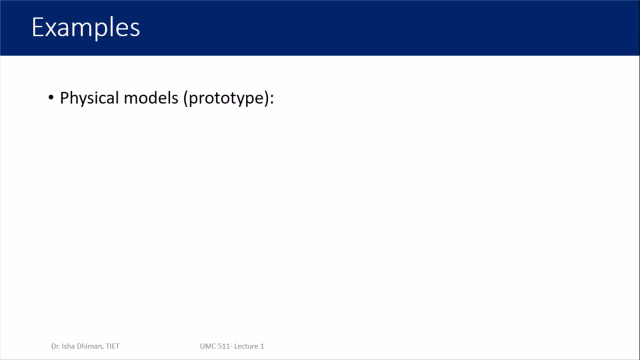 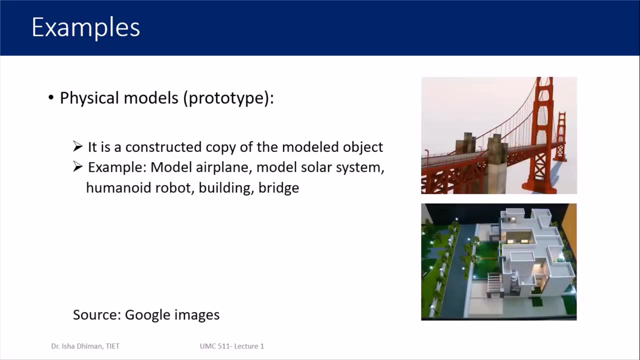 eyes, It is something which is nothing but a constructed copy of the modelled object. For example, it can be a model airplane, It can be model of a solar system, It can be a humanoid robot, It can be model of a building or a bridge. 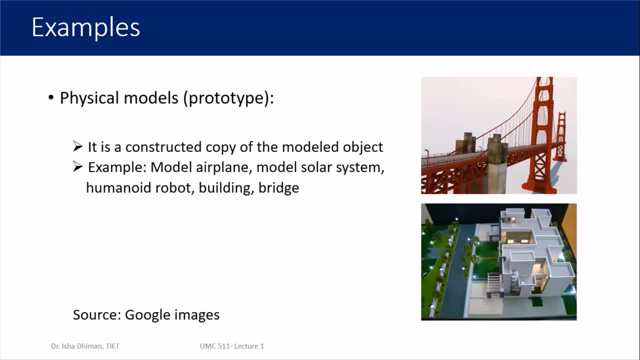 So these examples are very easy to find and this is having most of the time applications in thermodynamics, fluid mechanics, aeronautics and architecture. Obviously, this is not the exhaustive list. The list is much bigger than this, But this is just to give you an idea of what is the meaning of physical model. 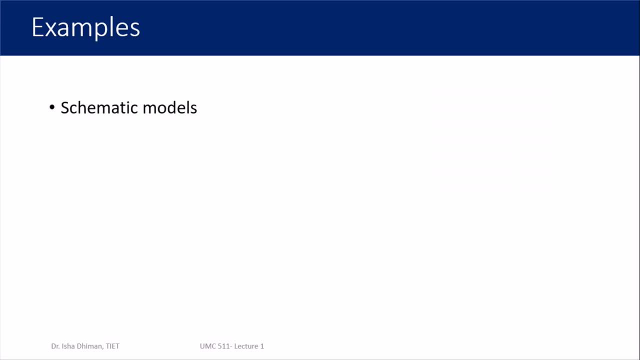 Next example we are going to look at is schematic model, And I hope this is also clear from the name of it. Schematic means the word schematic we use when we want to picturize something, we want to represent something through a schematic diagram or a graph. 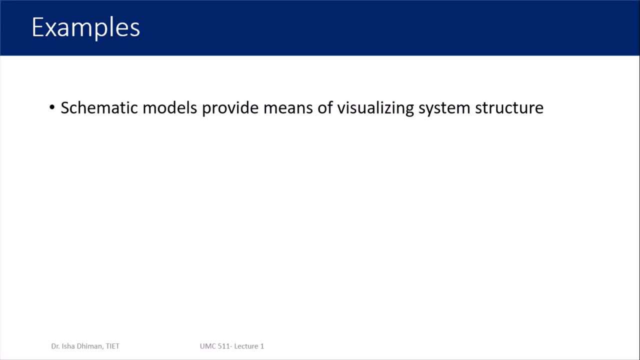 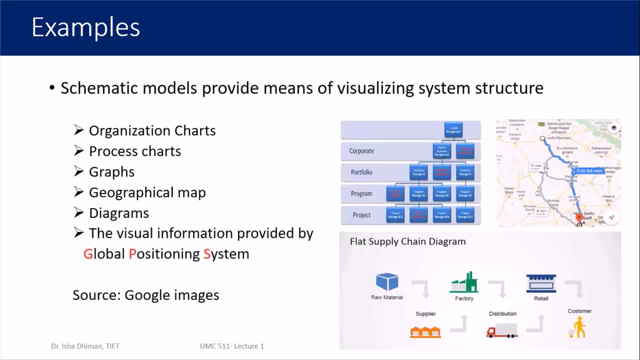 So this provide means of visualizing system Structure. So there can be many examples of schematic type of models. It can be the organizational charts, The process charts, graphs, geographical maps and the diagrams, And it can also be the global positioning system. 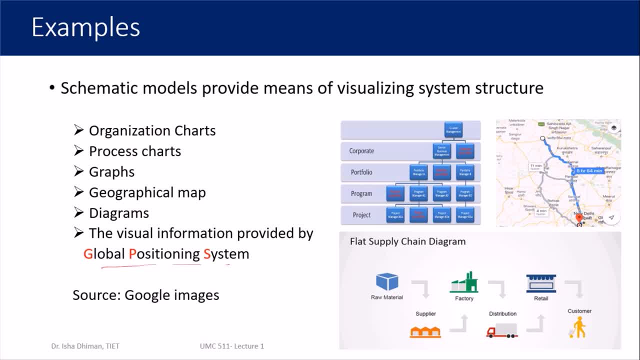 So the simplest example of a schematic diagram or a schematic Model is a geographical map. So you want to go from one place to another, Andольm i I, i am not familiar the route to be followed, so you'll take the help of a geographical map. 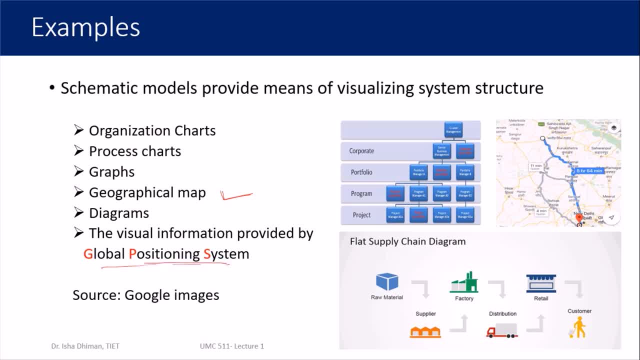 traditionally, or you will take the help of a GPS system. so the GPS is not going to actually show you the road. but if you look at this image over here on the right hand side, so GPS is showing you the schematic diagram. these are not the real roads, but the roads represented on the form of a picture, in the form of a. 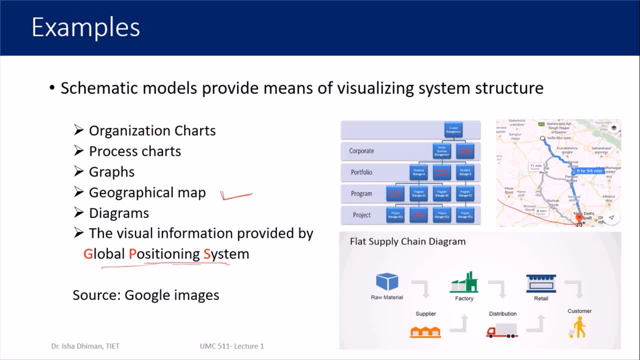 diagram or anything like that. similarly, you want to understand the structure of an organization, that who is the topmost, what is the topmost position in a company, and then what is the hierarchy of the company. so there are organization charts drawn. so the examples are plenty. you can think of your own examples, for 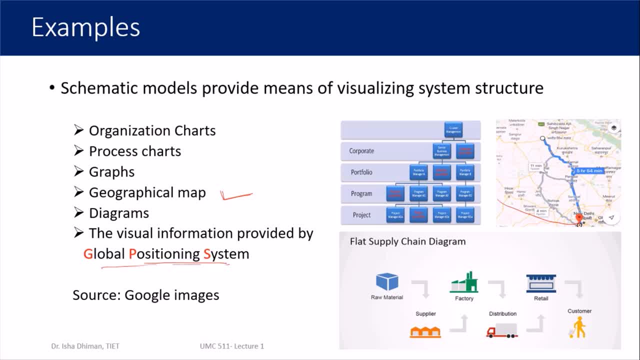 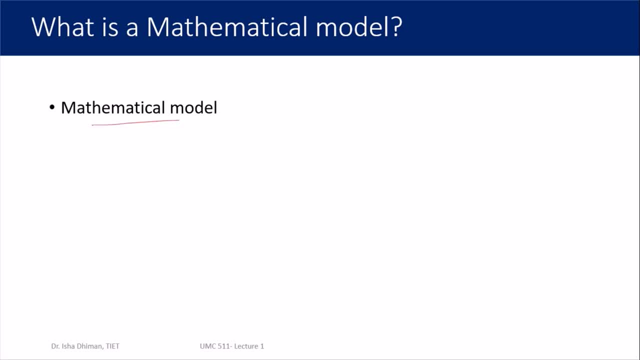 schematic type of models and now, specifically, we are moving towards our actual model and discussion, which is a mathematical model. so so far we have learned that whatever type of model you want to learn or understand, it needs a certain language. for example, the schematic model needed the language of drawing it needed. 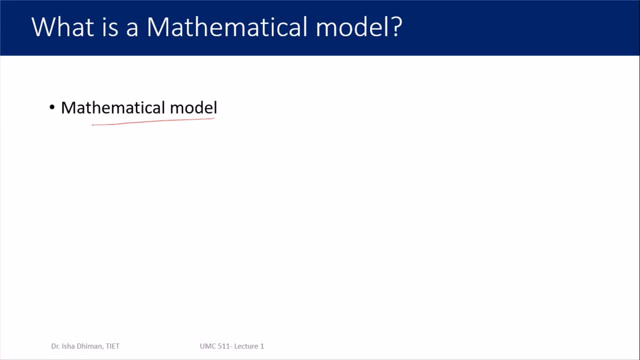 the language of visualization. similarly, a mathematical model is a representation of the behavior of real objects and phenomena in mathematical language. so the important word here is mathematical language. so we need to now think about this word, that. what do we specifically mean by mathematical language? so whatever comes to your mind when you hear the word mathematics is: 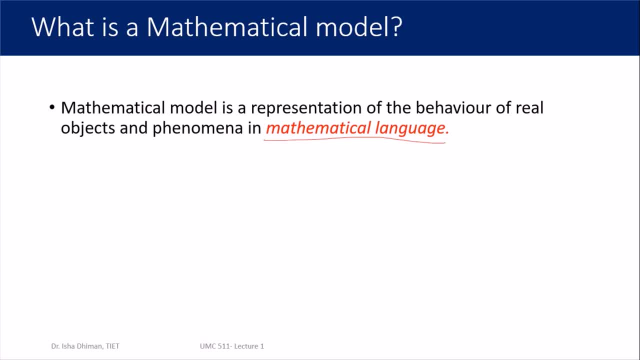 actually mathematical language. it is plus, minus, multiplied division, all those algebraic operations, elementary operations, square root, they are all the symbolic representation of mathematics and here we want to elaborate on the it to a bigger scale, So you can imagine you have algebraic equations. So an algebraic equation. 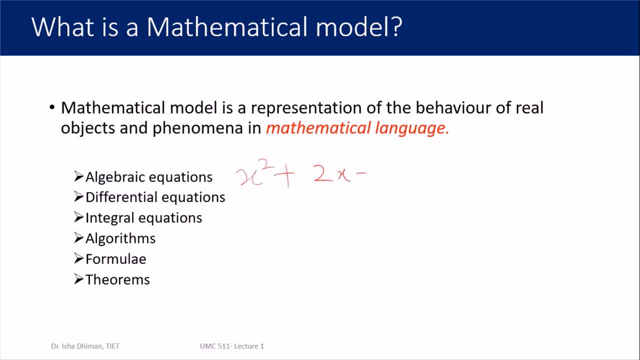 looks like. say you have this equation to solve means you want to find the value of x. So that means you are interested in solving this algebraic equation. The another example can be a differential equation. So all of us know how a differential equation looks like. So this is a very simple. 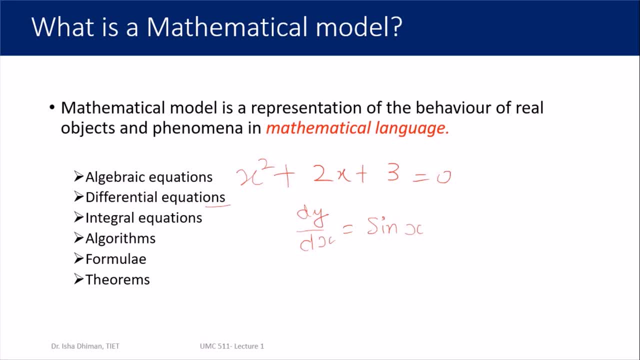 example of a differential equation. Similarly there can be integral equations, the algorithms or flow charts. They are also coming in the category of mathematical models, The formulas. so any formula like you want to compute the roots of a quadratic equation. So we know the formula is. 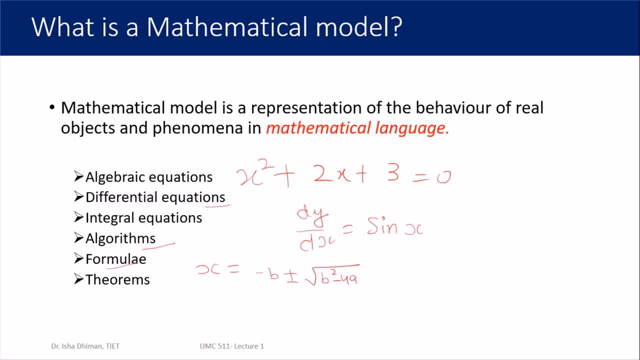 this. So this formula is also a certain kind of mathematical model. and the theorems and the lemmas, So whatever mathematical language you talk about, all of them are going to be in the category of mathematical models. So this is a very simple 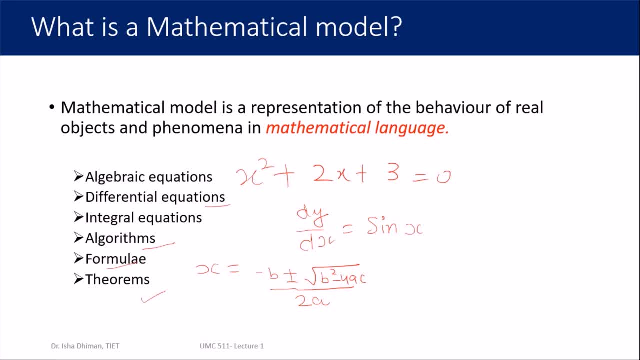 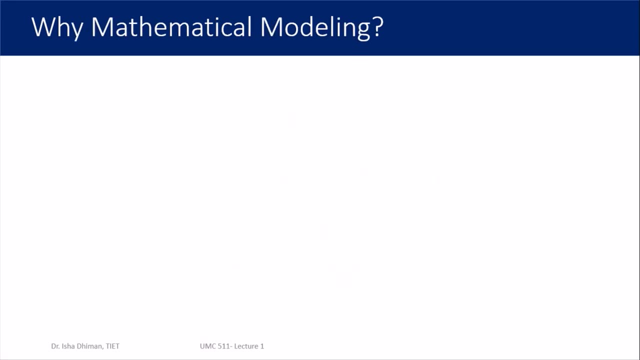 example of a differential equation. So all of these are one or other form of models. So I hope now we are clear with what is a mathematical model. and now we would like to move to our next question. We want to understand why we do mathematical modeling. What is the need of it? The world is 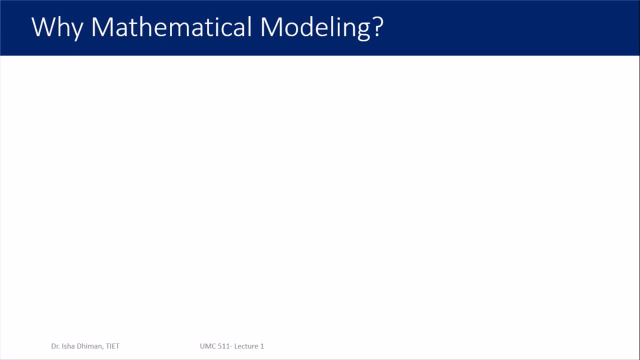 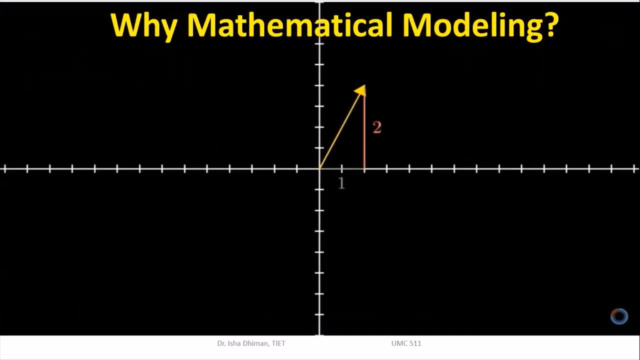 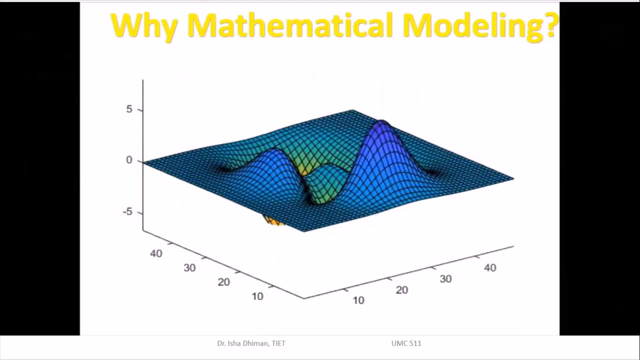 running itself Why we want to understand the things from a mathematical perspective. So the answer is: we know that all of us have been performing mathematical modeling, knowingly or unknowingly, since our school days. So whatever school level mathematics you have studied, whatever equations and formulas you have studied, ultimately they 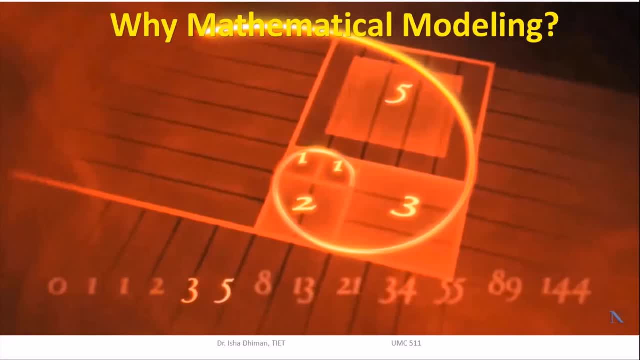 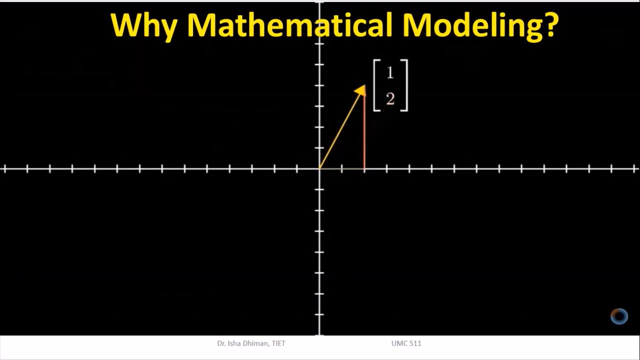 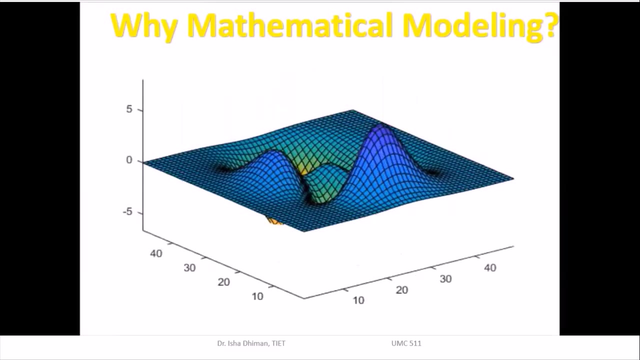 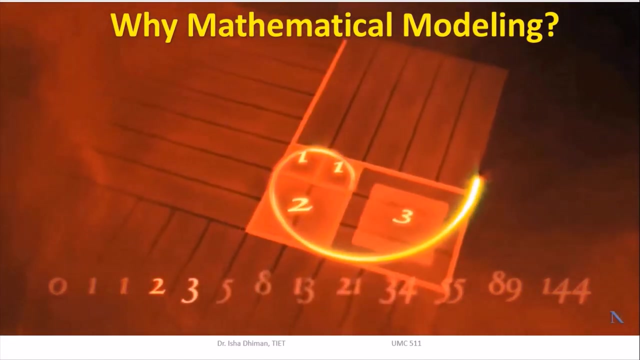 were nothing but all mathematical models. Many laws of nature are beautifully captured and explained with the help of mathematics, And even if you leave aside the aesthetic sense of mathematics, you will understand that there are many advantages of performing mathematical modeling. For example, there is no field of science and technology today which is untouched with. 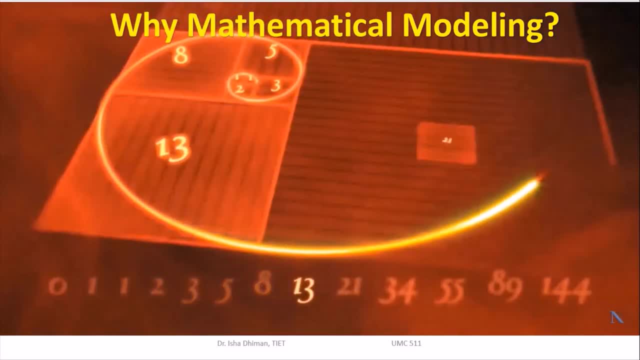 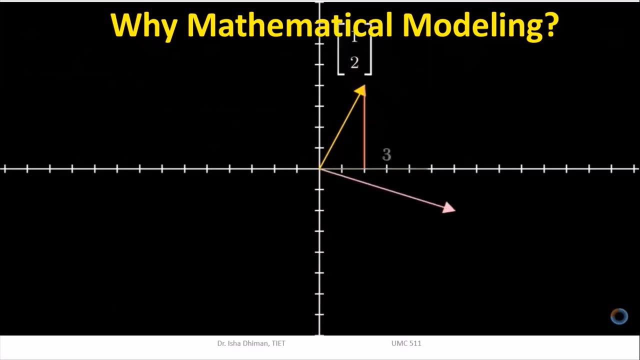 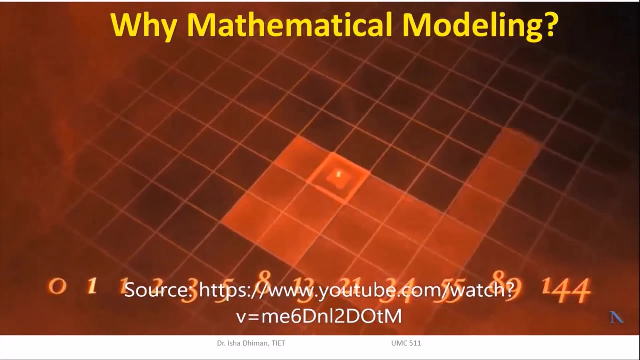 mathematics And, moreover, the best way to quantify the abstract behavior of some real phenomena. these words we will understand in detail when we go throughout the course. So the quantification of abstract behaviors. Abstract means something which otherwise cannot be measured or cannot be quantified. 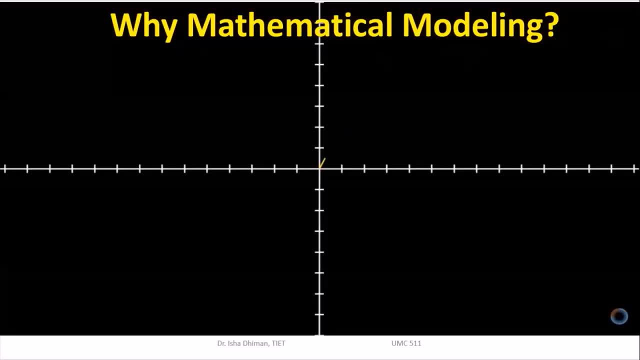 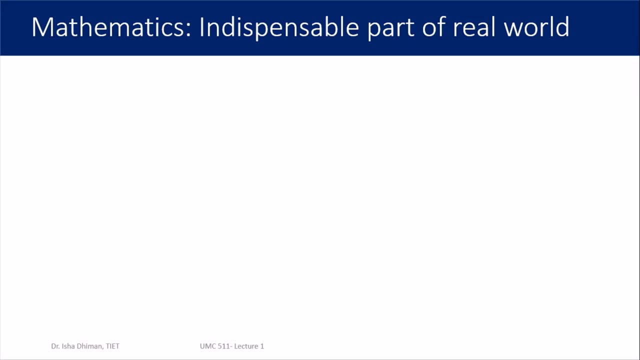 So the mathematical models make that possible. So there are many, many advantages of performing mathematical modeling and we will look at all of them. So that is enough for the motivation that why we want to do mathematical modeling. So now it's clear to us that mathematics is 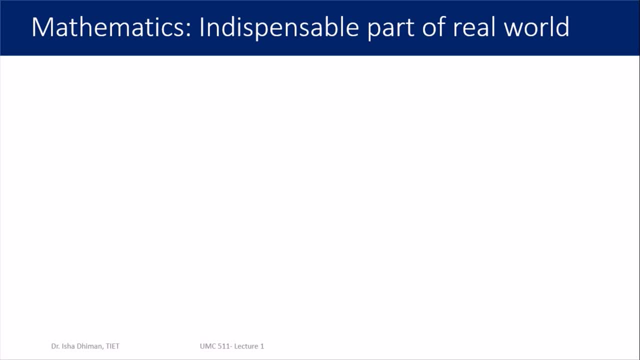 an indispensable part of the real world. Again, I would suggest you take a pause here and try to think of at least one example. Where do you think that mathematics is not used at all? or it is a real world, Or it is not connected with mathematics at all, And I know that you are not able to find any of these. 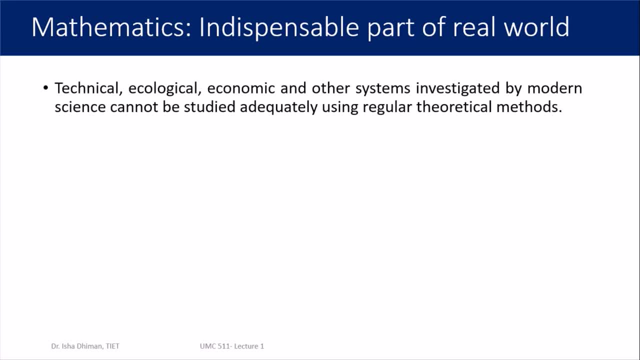 such examples like that. So to name a few applications, the technical, ecological, economic and other systems investigated by modern science cannot be studied adequately using regular theoretical methods, So we need to have some mathematical framework for doing that Direct experimentation. This is a very important point to understand. 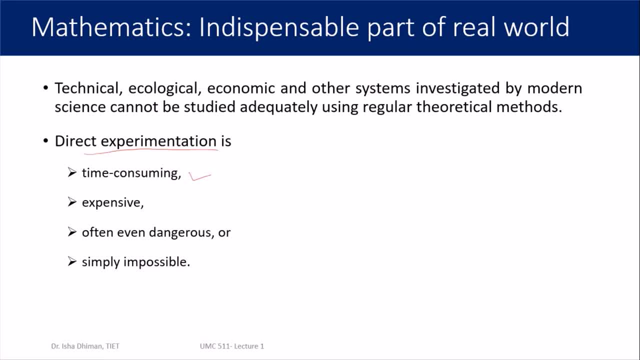 because direct experimentation is time consuming, expensive, often even dangerous, or simple or impossible. Because there are two ways of actually actually there are many ways, but broadly there are two ways of understanding any real phenomena. Either we want to study it theoretically, which I have just explained, that it's difficult to construct the theoretical. 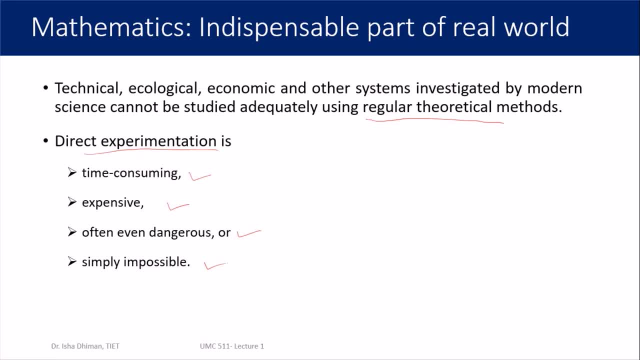 framework for each and every kind of real world phenomena. And the other category is we want to understand it through the experimentation. So here I'm telling you the limitations of performing experiments. The real experiments are time consuming and expensive, And in some cases it's actually impossible to perform the 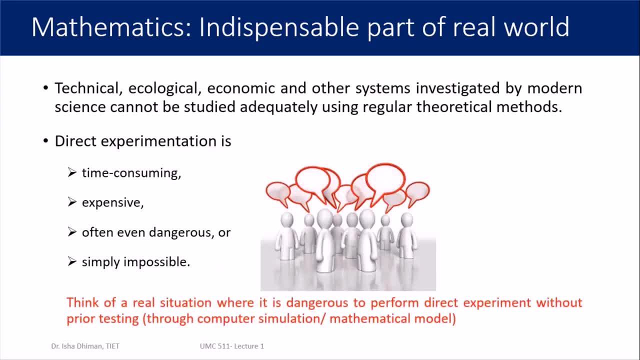 experiments. So you can think of a real situation where it is dangerous to perform direct experiment without prior testing. So even if you want to conduct experiment at a later stage, but still it is much more beneficial to do the calculations or the computations mathematically. 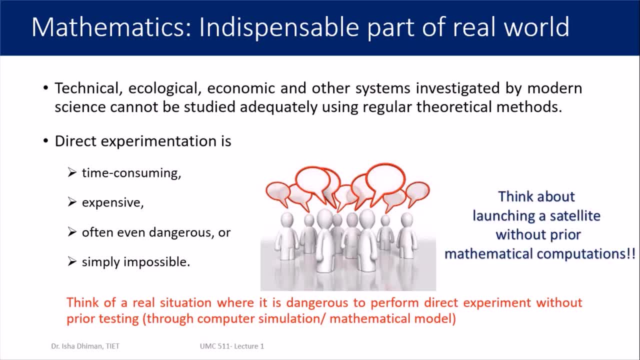 Prior to that. so you think of launching a satellite without doing any mathematical calculations and just guessing it, that this should be the velocity, this should be the trajectory to be followed, And so you better know the consequences. I need not say that. So that's just a very small example. It has much more higher level of applications. So 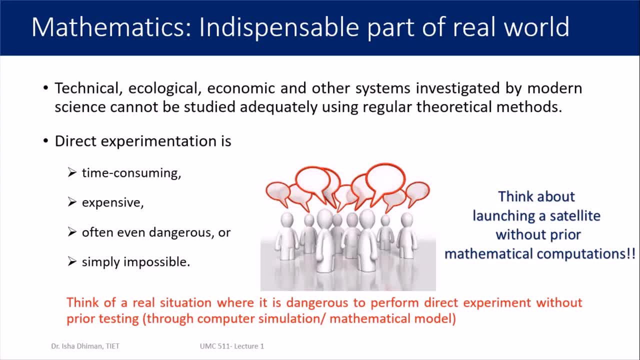 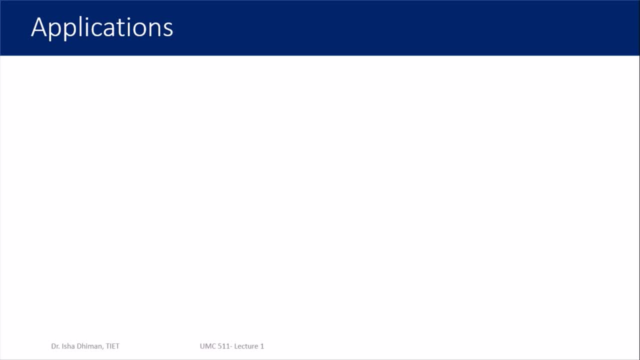 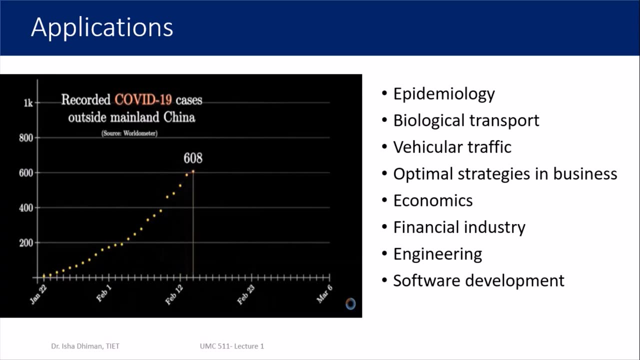 that's all about answer to the question why we are going to do the mathematical modeling. And now let's talk about applications. So again, the list is not exhaustive. I cannot really list all the applications here, but I've tried to cover the important ones. Epidemiology: Epidemiology is nothing but the 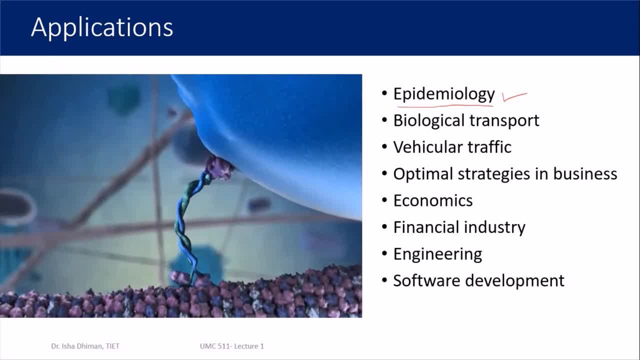 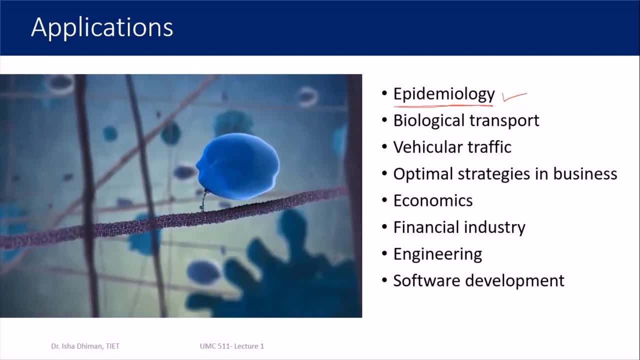 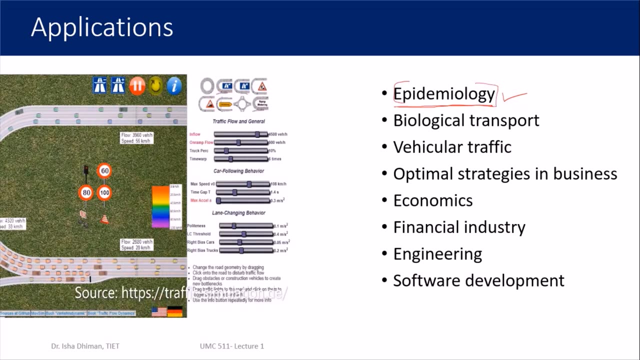 study of epidemics In the current times. if we are definitely not aware with the word epidemics, then definitely it's not worth it. All of us are already clear with the meaning of the word epidemics. So in the current situation of covid-19 outbreak, you know how much mathematics 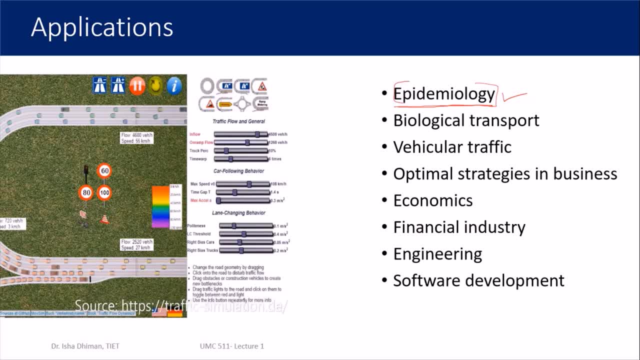 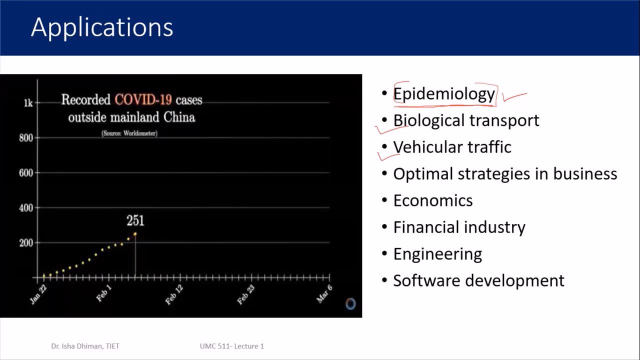 has been helping to understand the dynamics and predicting the curves and behavior of the virus spread. Another application can be biological transport and vehicular traffic. So here you can see a simulation of traffic, vehicular traffic running, and which you can see. Okay, So I'm going to show you now the application in the current scenario. So in the current 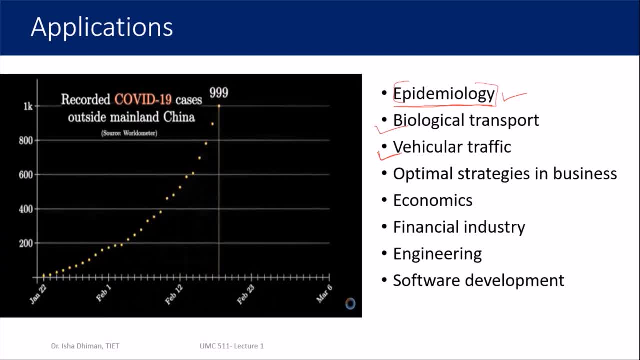 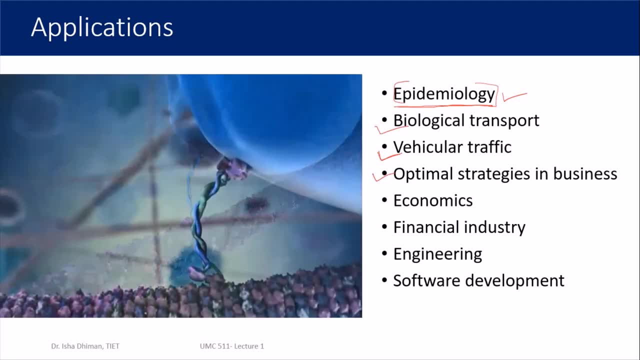 we will learn how to create these simulation models as well, so they are also coming under the category of mathematical models. and then, in business, you want to optimally. strategy is you want to decide your strategies optimally. for example, you have studied the course of linear programming, so they are in. 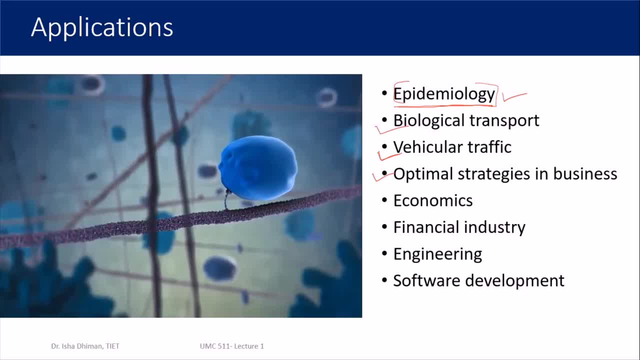 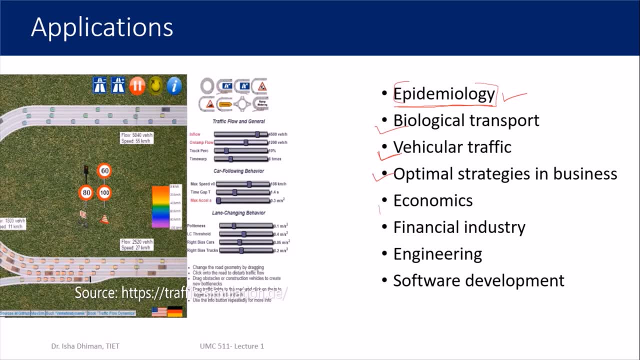 most of the business problems you are supposed to find an optimal solution. so that is also a linear programming. formulation is also a kind of a mathematical model. and then applications are in economics, financial industry will be talking about this in our course as well. engineering need not to tell you. 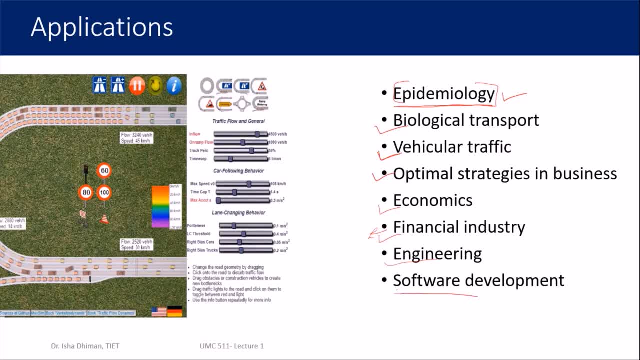 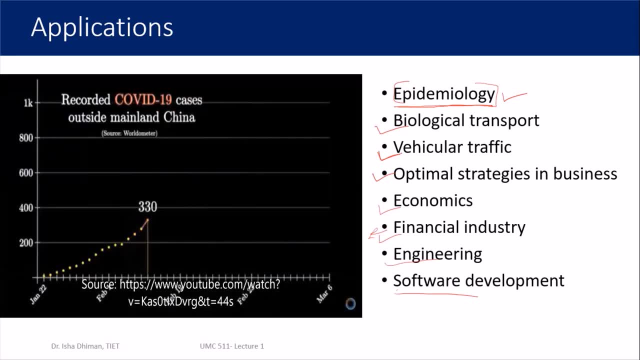 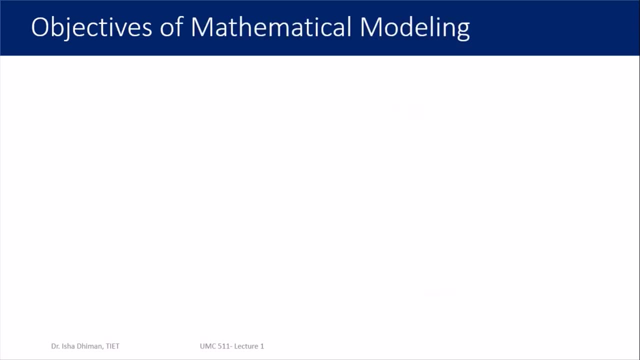 and software development. so these are very few applications of mathematical modeling. again, I'll tell you, you talk about an area and you'll definitely find an application of mathematics and the mathematical modeling. they are only so. now let's phrase: what are the objectives of mathematical modeling, what are the 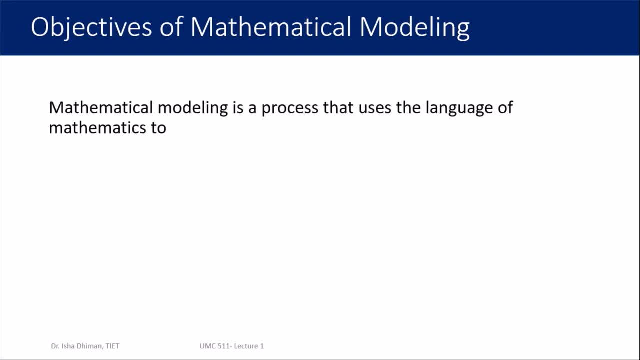 precise objectives of mathematical modeling. so the main objectives are: to analyze. we want to analyze something: why this is happening, how this is happening. if this is happening, then what are its effects, what are its causes? so that's the basic meaning of analyzing something: make predictions and then, based upon our analysis, we try to predict. just now I 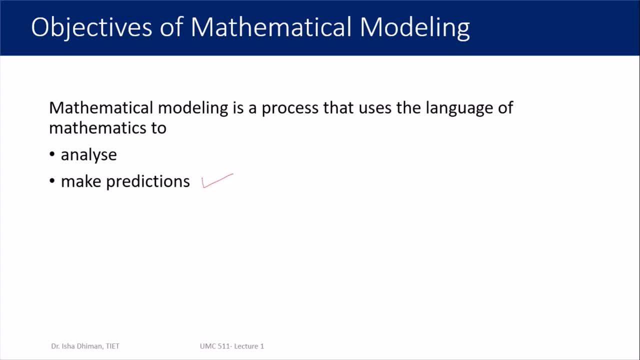 told you the example of this COVID-19 outbreak: the- looking at the trends, we want to make predictur. or you can have another example of stock market: that, looking at the trends, that where a particular stock is rising or falling, we want to make prediction for its future value, provide insight of the real-world. 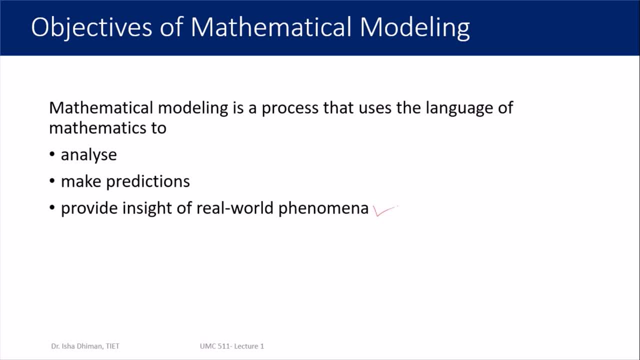 phenomena. so these are the main objectives of mathematical modeling. so not every model is developed to fulfill all of the objectives. some models are purely constructed for the purpose of analysis. some models are purely constructed for the purpose of analysis. so some modeling boundaries do not show the objectivepayers overall sense. this applies to bulbs. so these are theucci and deci-zons. these molecules are evolution. 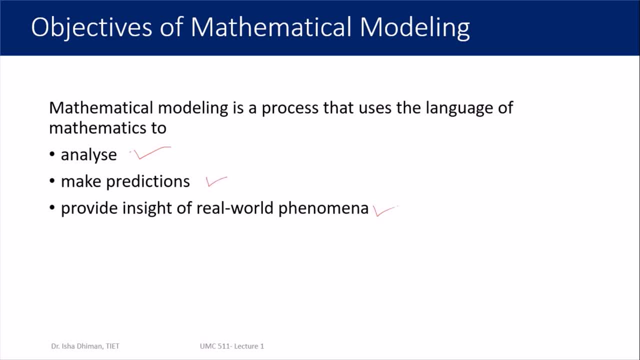 models are purely constructed for making productions- a weather forecasting model can be an example here, and some models are purely for this, and some models are there which cover more than one objective. so that will be eventually clear when we'll be studying different different examples of mathematical models. and, last but not the least, we also want to find optimal solutions to 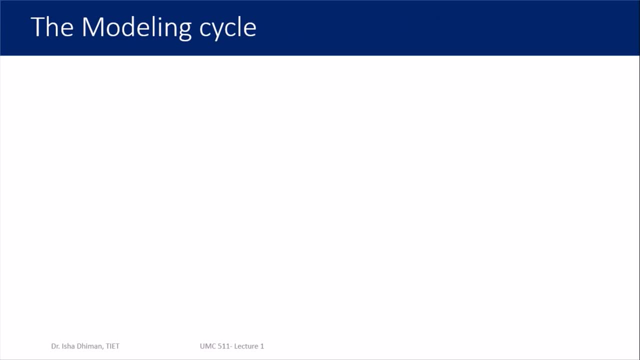 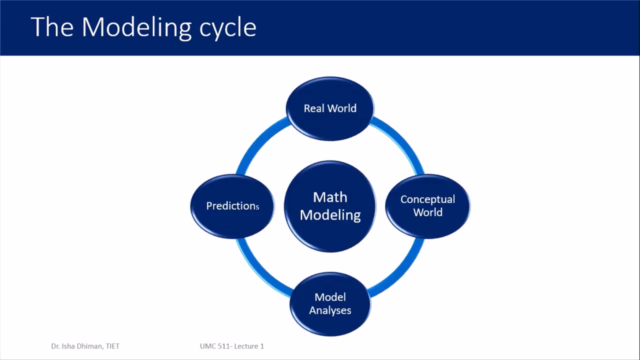 the real-world challenges. this also I have just explained to you. so now let me come to give you the definition of modeling cycle and you will understand after this why it is called a cycle. so this is a cycle because it starts from one place and ends at same place. so basically it starts from here, the real 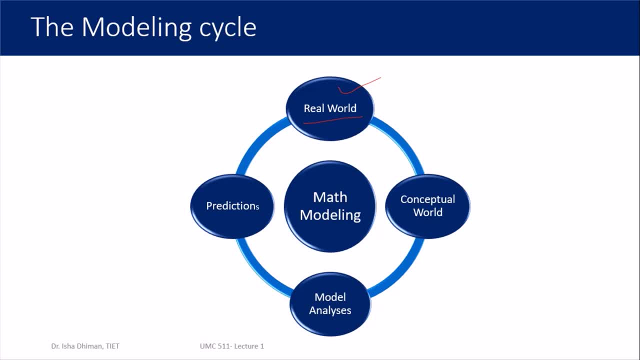 world. we are in the real world. we got to understand a phenomena so we actually move to the conceptual world. so here is the cognitive activity taking place, the real process we want to understand. we start to imagine that it in our mind, how it might be happening, why it might be happening or whatever we are thinking in. 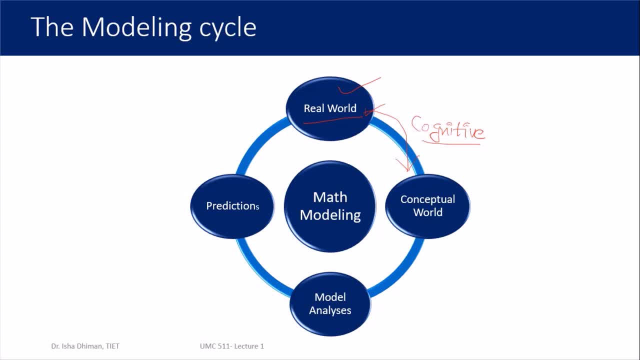 our mind. so basically, initial work of construction of model starts happening in our mind and imagination. that's why it's also said that modeling is a cognitive activity. so in the conceptual world we go. so what is the difference between the real world and conceptual world? so in conceptual world there are: 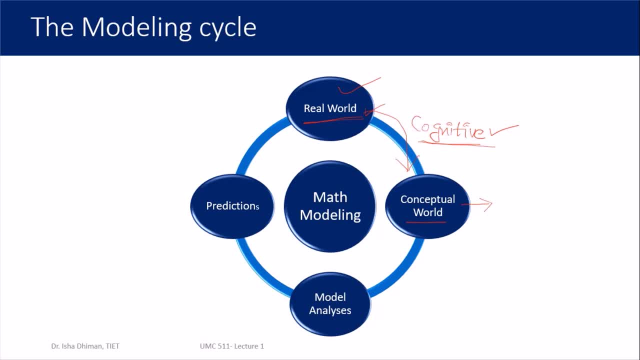 which are assumed, or there are some limitations, or you can say it's not a hundred percent exact representation of the real world. so, after conceptual world, we actually construct the model physically. we look at the model in front of ourself and then perform the analysis of it. after performing the 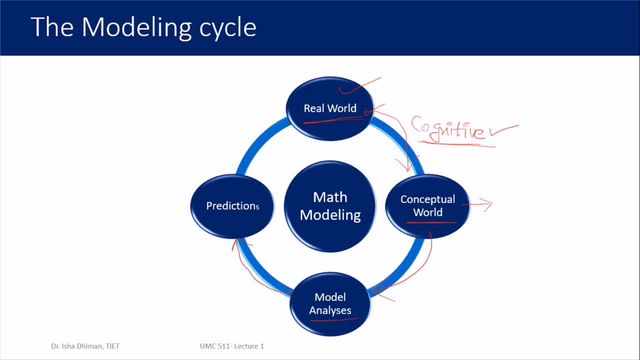 analysis, we predict or interpret the results and then these predictions we give back to the real world. so here also again to understand this example, you can have the example of this COVID-19 outbreak- that firstly we observe, okay, the outbreak is happening, the virus is spreading its infection. then we try: 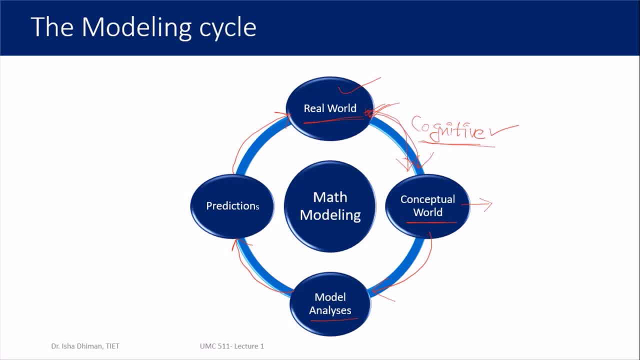 to think in our mind, okay, how this might be happening. this is coming from China, this is coming from there, and that, this, whatever might be the reason for it, and then we try to understand it mathematically, so we construct a model for it. study in our course some epidemic models, and there will be talking about 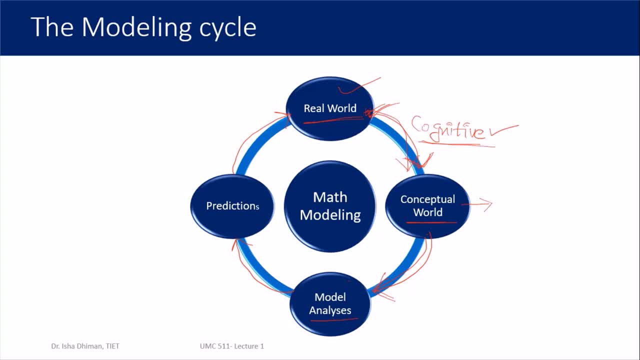 these models in detail. so after construction of model, we gets some answers: okay, this is going to rise, this is going to decrease, this is going to happen. so those results are mathematical. and then, to make the predictions understandable to the layman or to the real world, we interpret the. 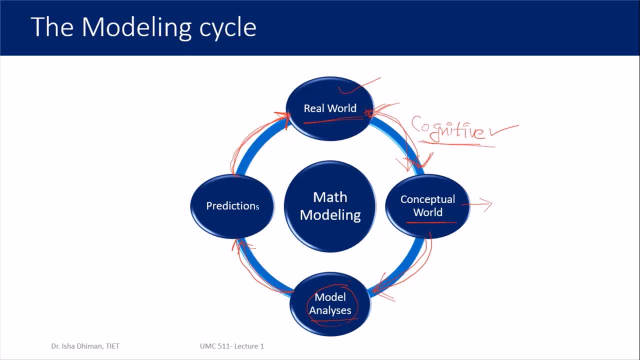 result back in the language of real world. so the mathematics again gets related to the language of the real world. so that completes the cycle of the process which is called math modeling. so that's the meaning of this modeling cycle and that's why it's called a cycle, because we started the real world and we 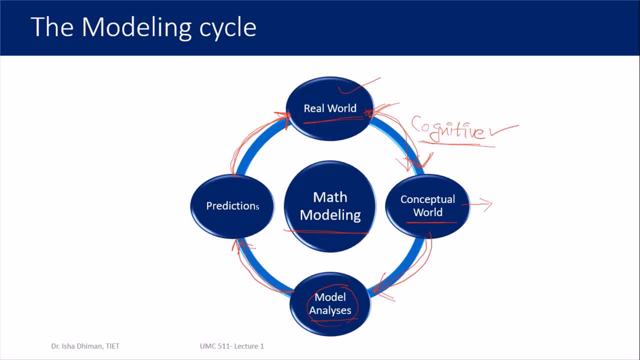 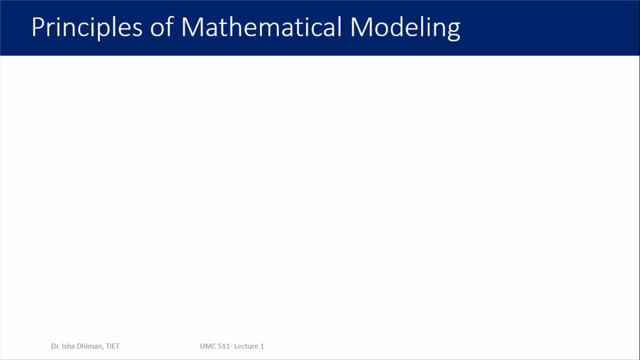 end at the real world. if we do not complete the cycle, then the process is considered incomplete. and now we'll move towards the understanding, the principles of mathematical modeling. although you will see that each model is a different kind, is it is distinguishable from the other one? it is. 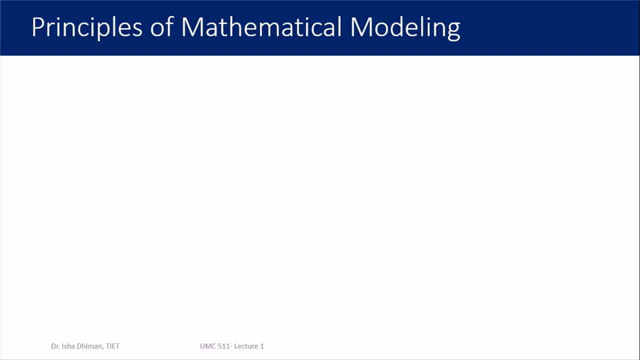 having different characteristics, but still there are some commonalities in all the mathematical models and which are known as the principles. so you can understand. these are the fundamental rules which we have to follow in the process of mathematical modeling. so basically, there are four major steps: the 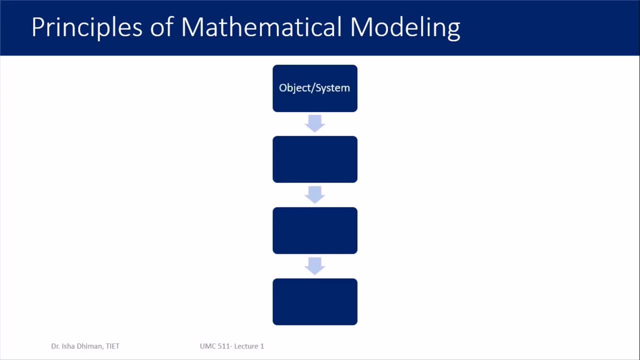 first is we have to identify: identify the object or the system which we want to model. so here, basically, what we are going to look at is we are going to redefine our purpose, why we want to understand, like i explained you, that there are many objectives of mathematical modeling. we should be clear with what particular 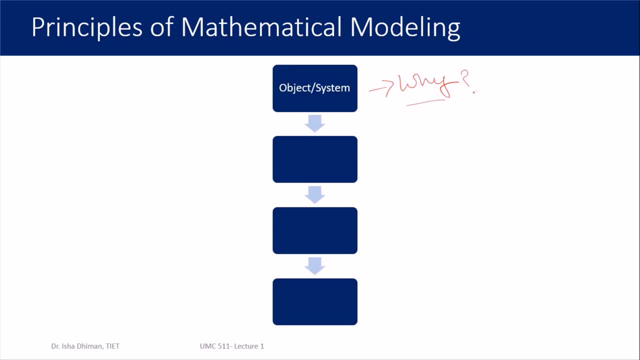 objective i am performing the mathematical modeling- why you are constructing this model, you want to analyze it, you want to use it for prediction or you want to do something else with it. so that clarity is very important here: that why we are doing so and then what we are trying. 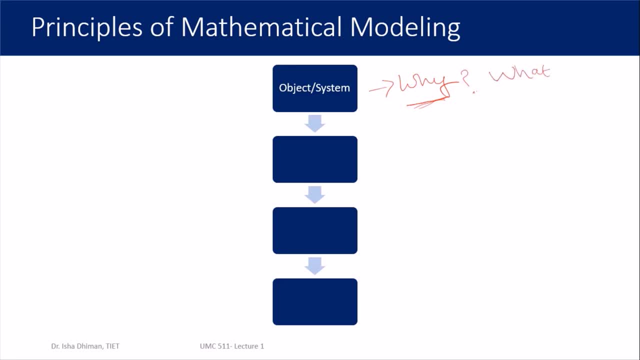 to achieve. that's basically the same thing, what i've just explained you. so that means here, after identifying the real life object, we want to define our purpose. so once we have thought that so, then we will follow the process of mathematical modeling. so, briefly, i have just explained you the process of 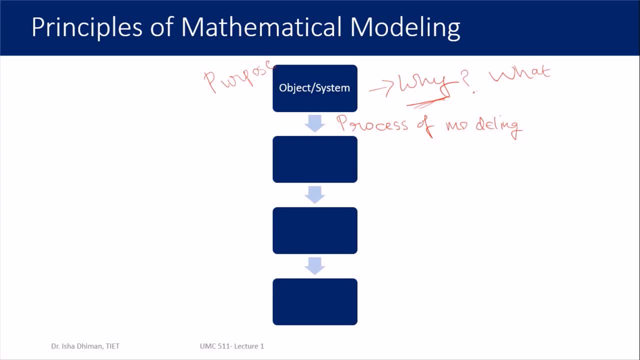 mathematical modeling through the modeling cycle, but we'll be talking about this process in more detail in our next lecture. so here right now, you just assume that some process is happening, some number of steps are happening here to go towards the next step. so, after doing this process of 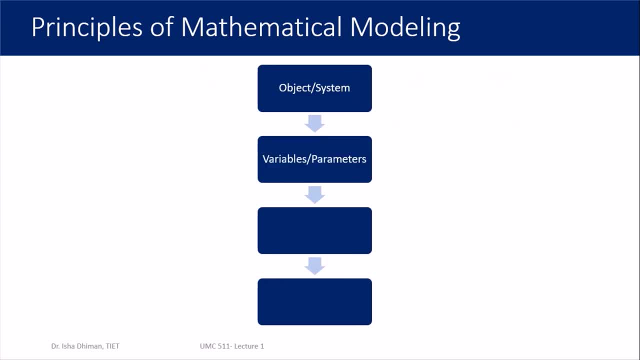 modeling complete, we get to actually look at the process of mathematical modeling. so we are going into theTuF model and i'm really doing an all-ундance analysis and then talking more about other France, democratization and other countries, and i will leave you with this어�. 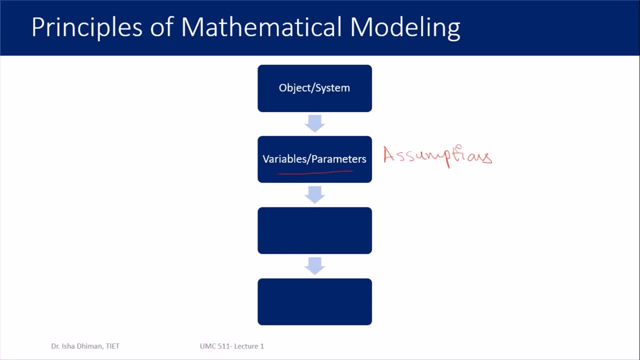 on some. ﷺ. this is justド. let's break, go to this model. first step. what are we going to do now? let's talk about it. this is just the negatives here. i want to calculate, just to count this, how much time we have time to do we not now? why do we think this, if we feel like d2i and d3es is the actual way we can? actually we're not英 job numbers like that. i always think we're not being able to mapweh, and i just wanted to clear the links in my head. furtherord. 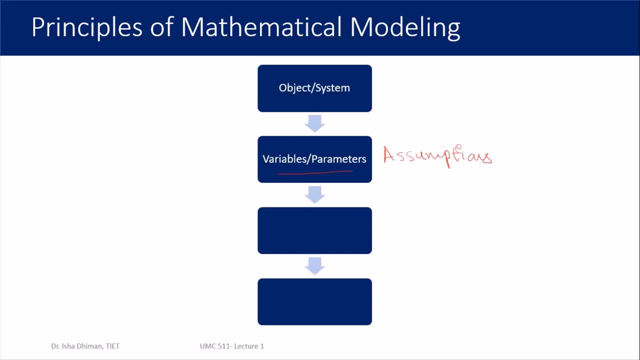 in fact we know that we make a simplistic version of that and for that I have to lay down certain assumptions. so that's the first step. we have to define some assumptions for the variables and parameters. we want to define that. which parameters effect we want to see again take the example of this virus spread. so you want to. 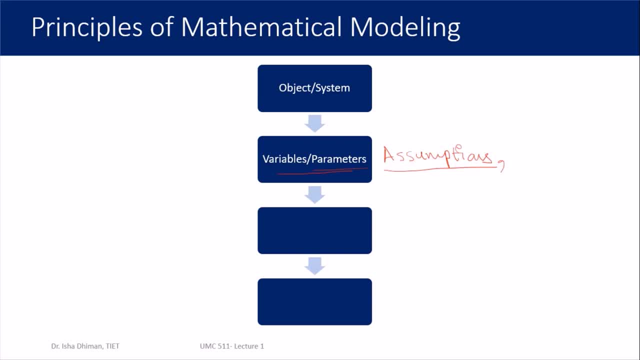 understand how the virus is spreading. so it will depend upon what kind of study you want to conduct. you want to study the effect of temperature, or you want to study the effect of gender bias, you want to study the effect of age groups. so, whatever parameter effect you want to study on that particular model that you 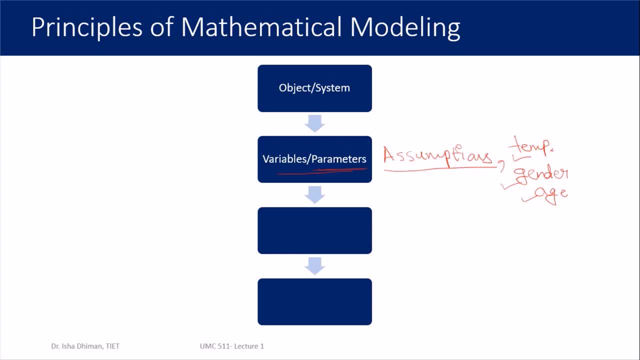 will be redefining here, so the model is constructed up to this step, and then what we are going to do is we will solve this model, because this is that stage where you already have some maths into the picture, you have some equation, you have some expression in. 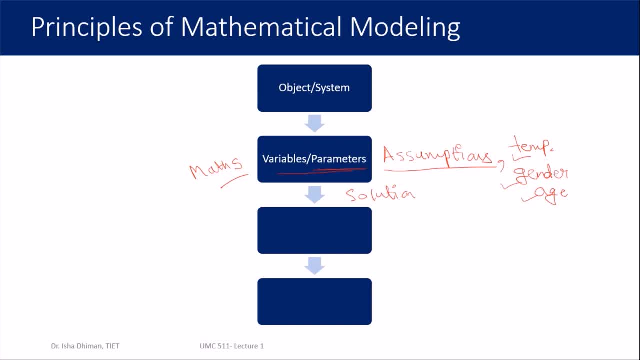 front of you. so, depending upon what it is- differential equation, integral equation, algebraic equation, system of equations- so it can be anything, we will solve it. so the question arises: how to solve it. so there are two ways: either we can solve it analytically or we can solve it. 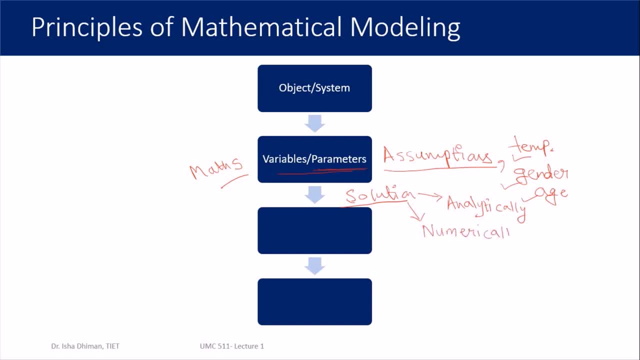 numerically. Again, we'll be talking about the solution techniques, depending upon what type of model we are studying. So I'll be just not going to detail at this stage right now. So, whatever way you solve it, you have the solution at hand. So once you get the solution, then we are going to. 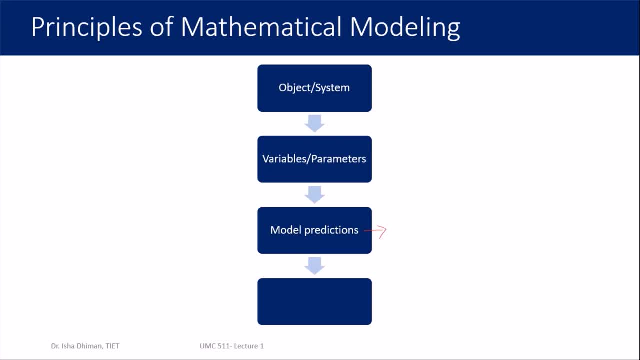 get the predictions that what information this model is giving us. So we will interpret our mathematical results in the language of real world. We'll give some outcome that, okay, our model is telling that the virus is going to spread its effect with a this much rate or that much rate. 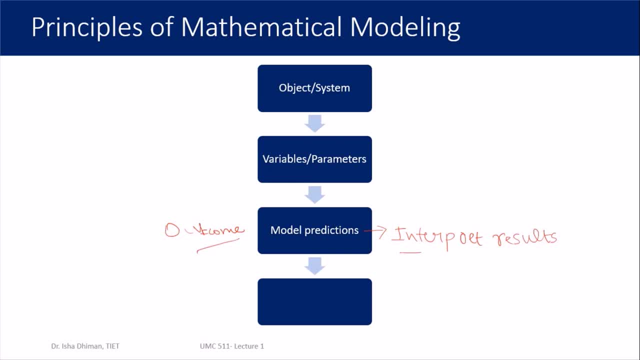 whatever is a mathematical outcome. So we will interpret our results and then, after giving the results, we cannot just stop there. We have to see whether the result is coming out to be valid or not. So there are two possibilities here. So firstly, we need to perform the step of validation. 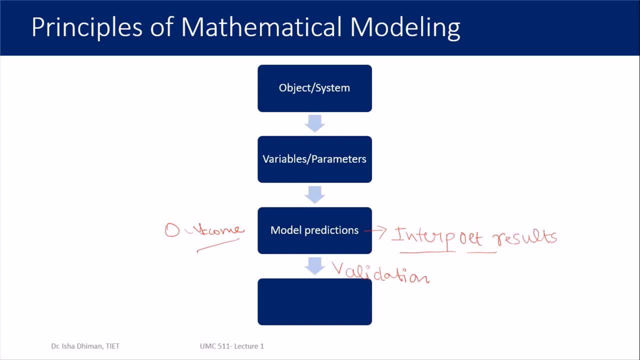 So the process of validation is further depending upon how you are doing the validation or what particular model is with you. Sometimes the validation is done through experimentation. You have the experimentation data, you have the experimental data, You verify the outcome at joint experimental data You prove that that particular story is correct or false. 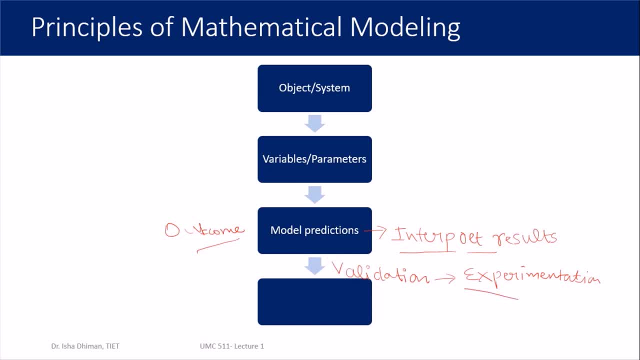 So now you are going to perform your evaluation. First step is to go back to the initial implementation of your model with the experimental data. so if they matches, so that means your model is working right. and sometimes the validation is done intuitively. intuitively means you need to understand the laws of physics of the model there. 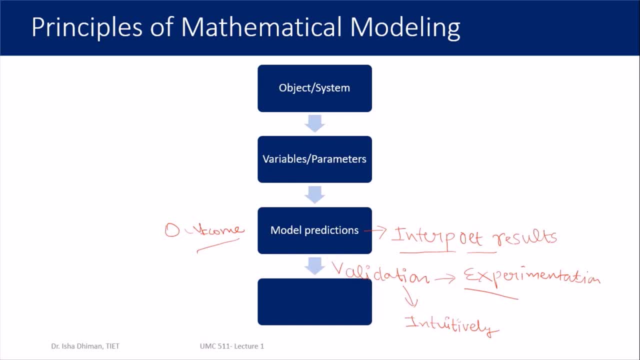 that, whether the physics of the model is right, in the real world, whatever should happen is happening in the model also, or not? for example, say, in some population model, the final answer of population is turning out to be negative. so obviously a negative population is not a well-defined quantity. it's